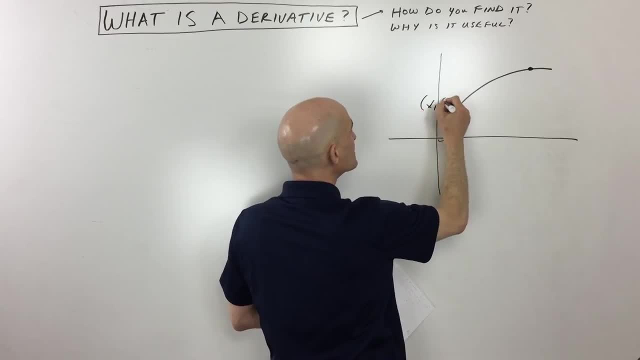 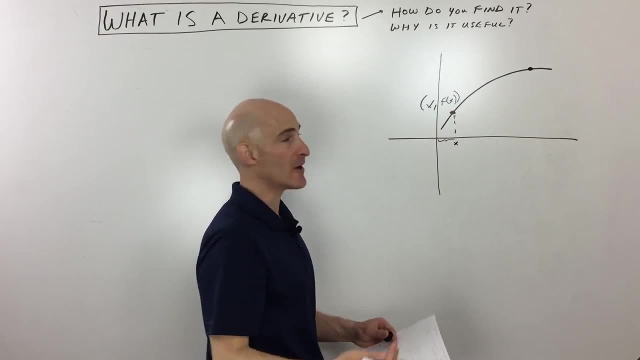 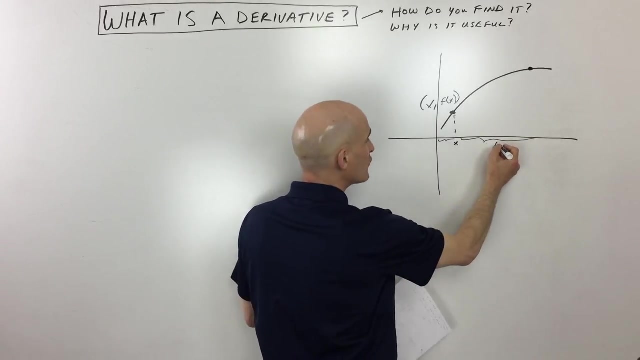 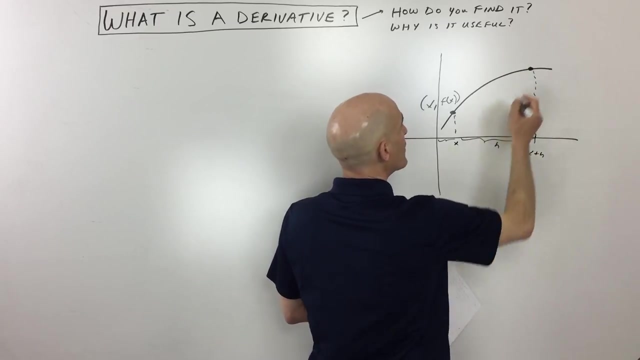 go up to our function. this point here is going to be x comma, f of x. Okay. so when you put that x value into your function, you get out the y value or the f of x value right Now. if we go a little bit further to the right, okay, let's just call this distance h. Okay, so you're with me. so far. That means over here we're going x plus h. okay, x plus h. And if we go up to this point on our graph right here, we've got x plus h. if we put that into the function, the 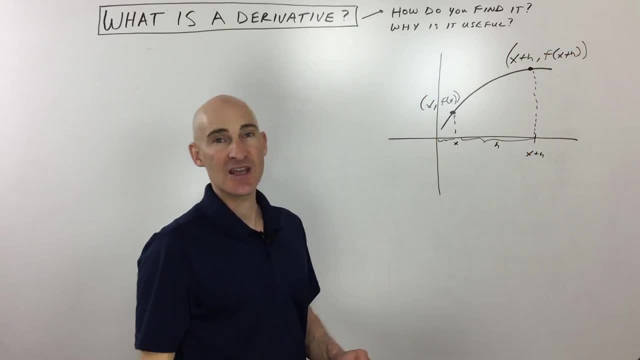 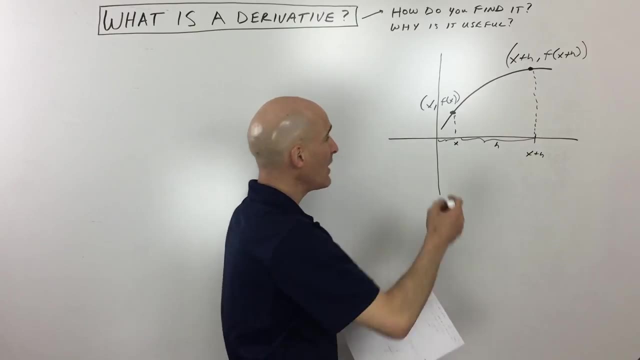 output, or the y value, is f of x plus h. Okay, so all we've done is we've just written this in a real generic way, But what we have is we have two points on our curve And now what we're going to do is we're going to find the slope, Okay, between those two points, Okay, And when you find the slope, remember your slope formula from algebra- it's y2 minus y1 over x2 minus x1, right, That's our slope formula. In this case, it's going to be f of x plus h. 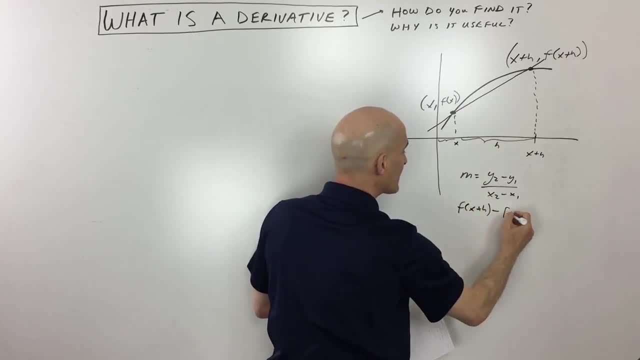 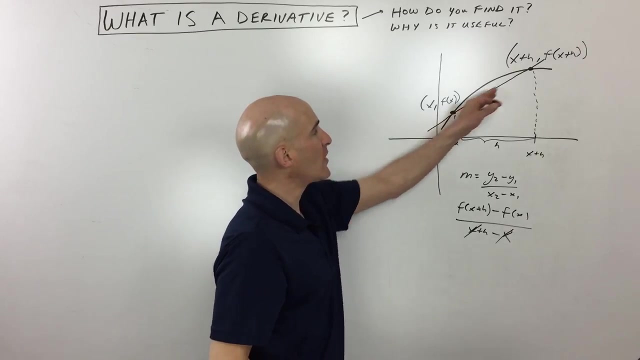 Okay, that's that y value minus f of x right, divided by x2 minus x1.. So that's going to be x plus h, okay, minus x. And you can see here that the x plus h minus x, right, you can see that the x's are canceling and we just have each in the denominator, right. But now let's take this a step further. So what we're doing right now is we're actually finding the slope between these two points, which is the average rate of change. Okay, it's this. 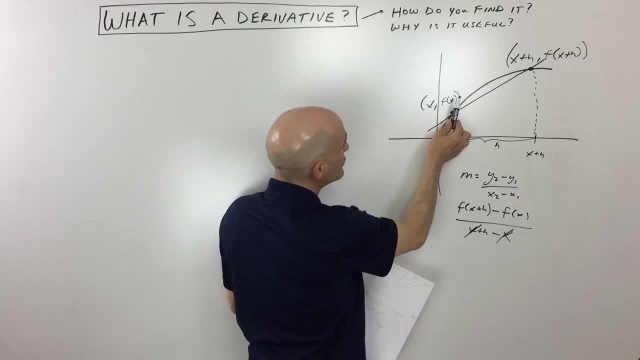 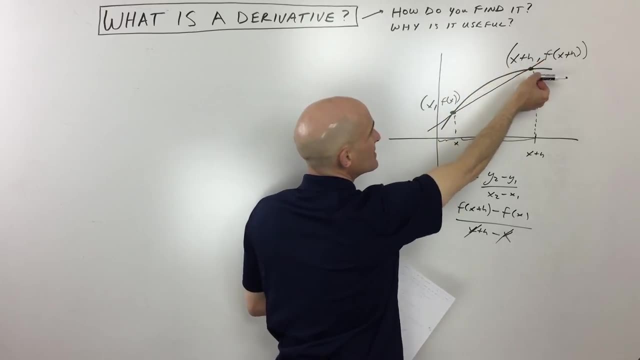 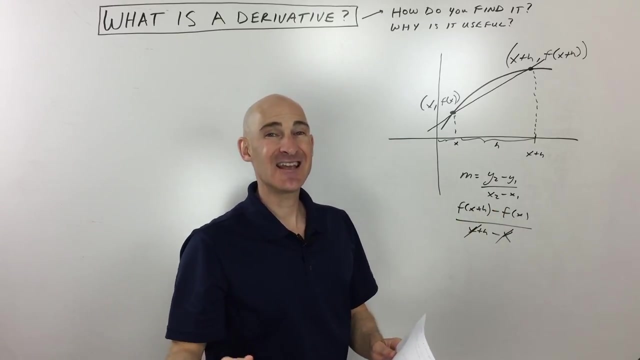 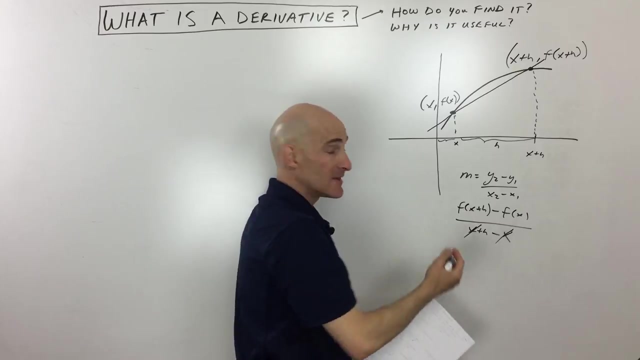 average slope, But you can see that anywhere along this graph the slope is constantly changing, like here: okay, it's at an angle like so, Here it's a little bit less steep. Here it's even less steep. Here it's even less steep. Here it's even turning around and going the other direction, right. So what we're doing is we're finding a formula for the instantaneous rate of change- okay, the slope at any point along this curve. And the way we do that is we introduce limits and it's the limit as h approaches zero. What that means is: 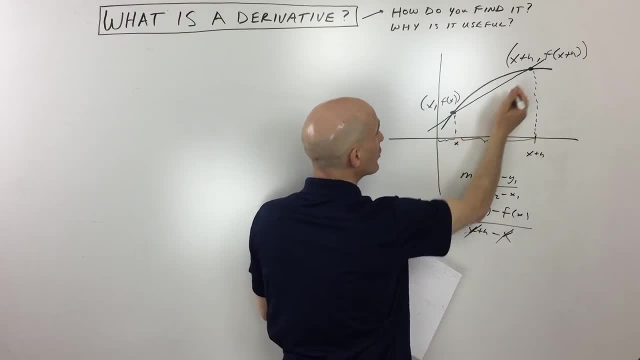 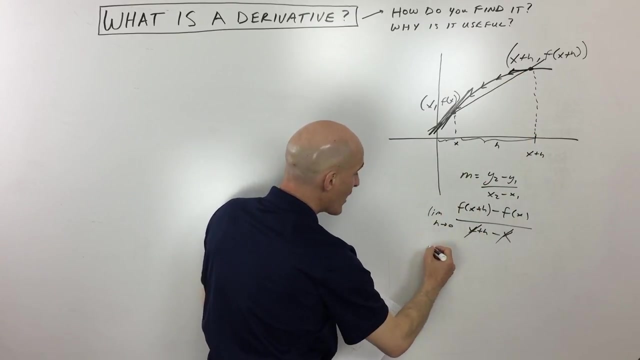 as this distance right here gets smaller and smaller and smaller. this point here, in effect, is moving along this curve until these two points are right on top of one another and that distance is zero. And so what we're getting now is we're getting the instantaneous rate of change instead of this average rate of change. So what you're seeing right here- and let me just rewrite it a little bit- is this is the limit, as h approaches zero, of f, of x plus h. 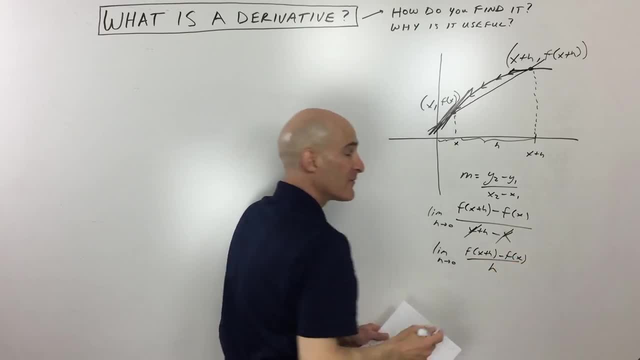 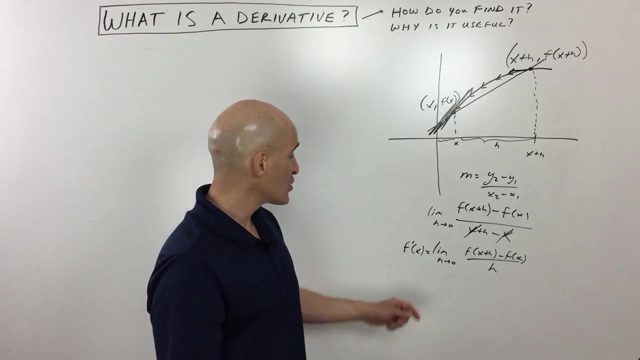 minus f of x, all divided by h. This is referred to as the difference quotient. Difference, remember, is subtracting, Quotient is dividing, So altogether they call this the difference quotient. But when you get to the end of precalculus, beginning of calculus, they start to refer to this as f prime of x, which is the derivative. So don't get confused by the word derivative, It's really just a formula for the slope of the tangent line, okay, the line that just barely touches that graph at that one point. 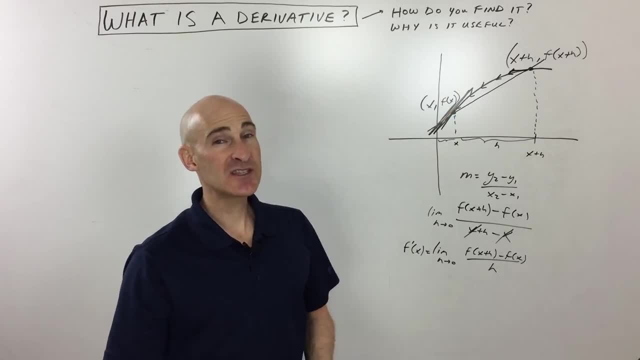 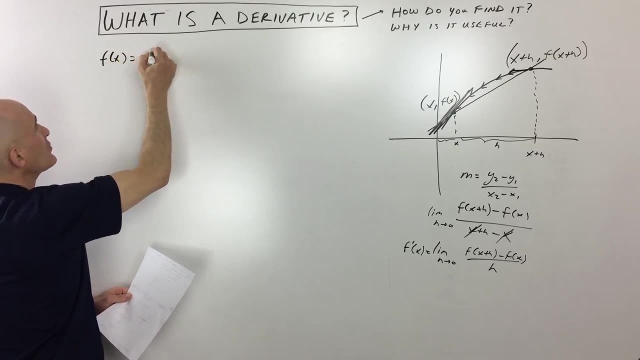 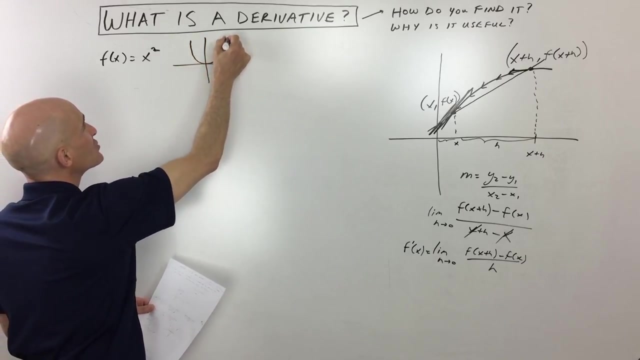 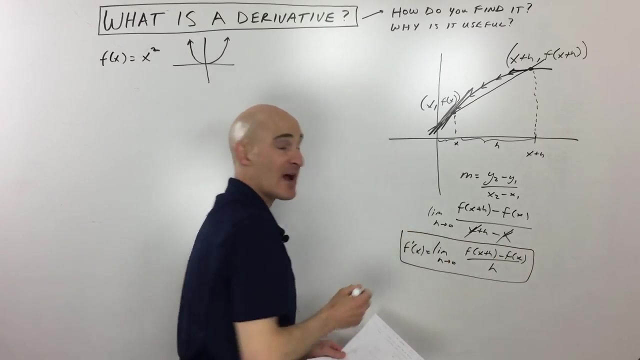 And it gives us the instantaneous rate of change. So let's get into a basic example now. Say, for example, your function is like this: f of x equals x squared. Okay, so we've grown up as we've gone along in math and we know what f of x equals x squared looks like. It's just a parabola, like: so right. But now what we're going to do is we're going to use our derivative. we're going to use our difference quotient to find the derivative, okay, which is a formula for the slope of the tangent line at any point. 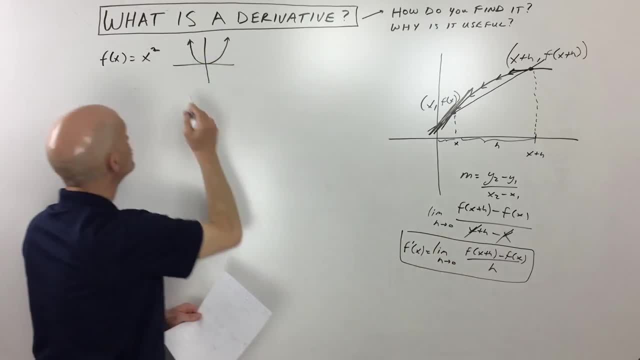 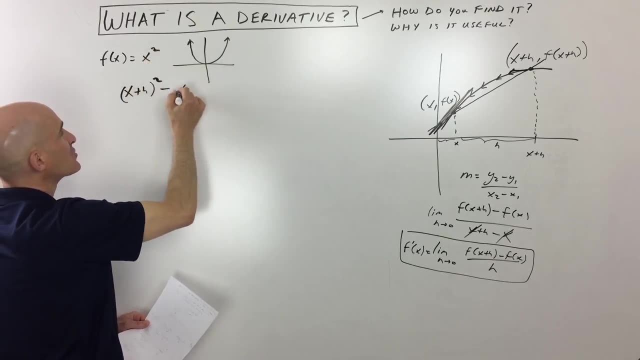 At any point along this graph. So what we're going to do is: let's go ahead and do these substitutions. here We're going to put in x plus h, okay, squared minus f of x, which is the original function, that's x squared all divided by h. So if we simplify this, we get x squared plus 2hx plus h squared minus x, squared all divided by h, And it's the limit, as h is approaching zero right Now, notice that the x squareds are canceling each other out, And then here we can factor out an h, which 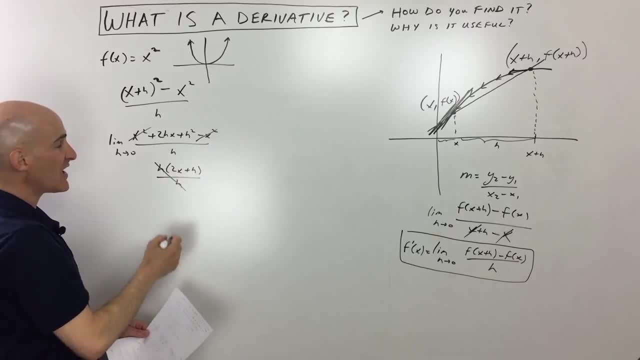 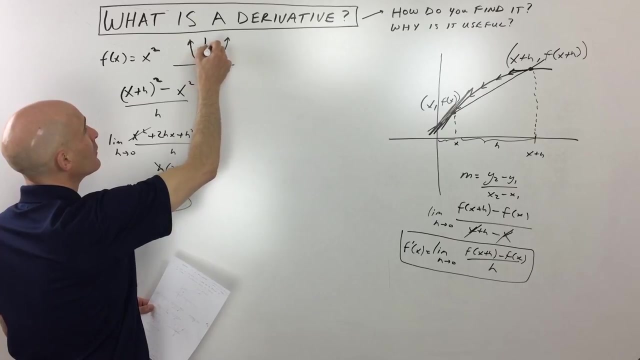 gives us 2x plus h, all divided by h. So those h's cancel And again, remember, it's the limit as h approaches zero. If we put zero in for h, we're left with 2x And this is our formula for our derivative which, remember, the derivative- is just a formula for the slope of the tangent line. So a simple example would be say we were interested in finding the slope at the point 2,, 4, okay, right there, Okay, so we're trying to find the slope of that tangent line. Well, if we put in that, 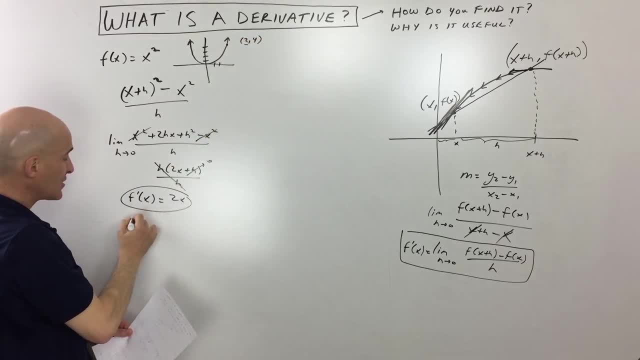 x coordinate 2, okay, in for x here. that's going to be f prime of 2, which is equal to 2 times 2, which is equal to 4.. And again, remember, this is a formula for our slope. So now we know that the slope is 4, and it goes through the point 2, 4.. Let's write an equation of the tangent line. So that's going to be: y minus y1 equals m times x minus x1.. We're just going to use the point slope form. So this is going to be: y minus 4 equals the slope, which is also. 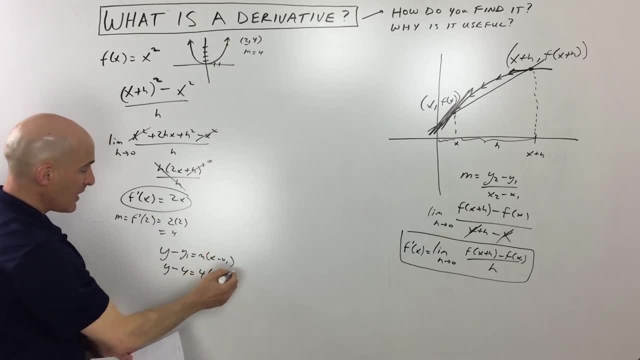 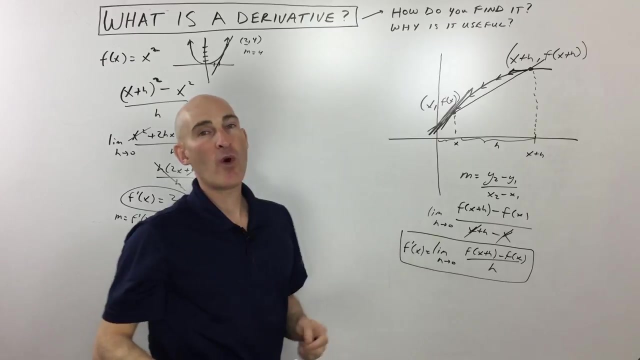 4 times x minus the x coordinate of the point, which is 2.. And that's an equation for our tangent line. okay, like so. Now let's get into another example about you know, we talked about how to find it, we talked about what it is and another example of why it's useful. 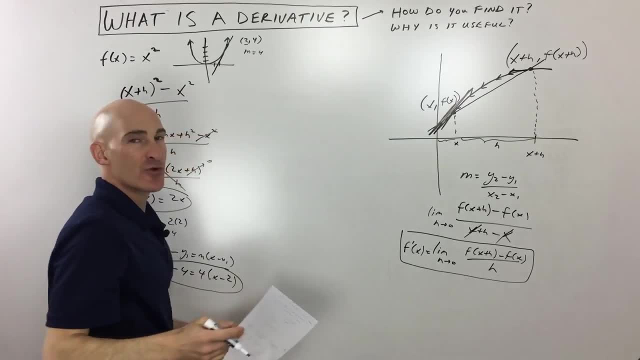 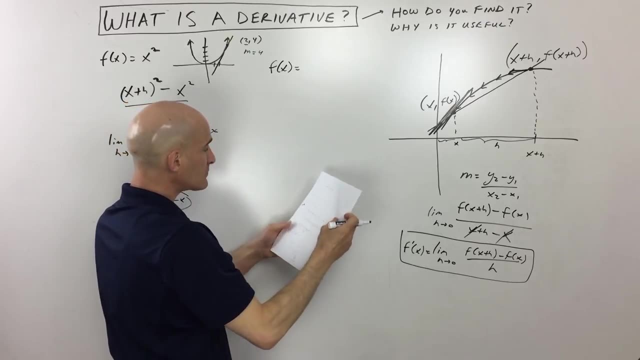 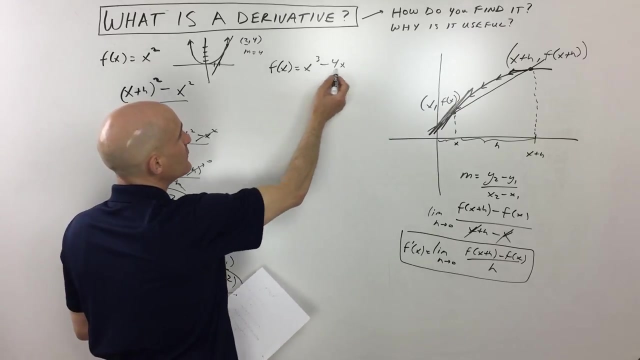 So you probably remember from Algebra 2 and Pre-Calculus when you were graphing polynomials. So take, for example, this polynomial here: f of x equals x cubed minus 4x, right? So one way we would graph this is we'd say: all right, let's see if we can factor this and find the zeros. Remember, the zeros are just the x intercepts. So if we factor this further, we get x plus 2, x minus 2, bring down the x. If we set all these factors equal to zero, you can see what we're getting is we're getting zero. we're getting 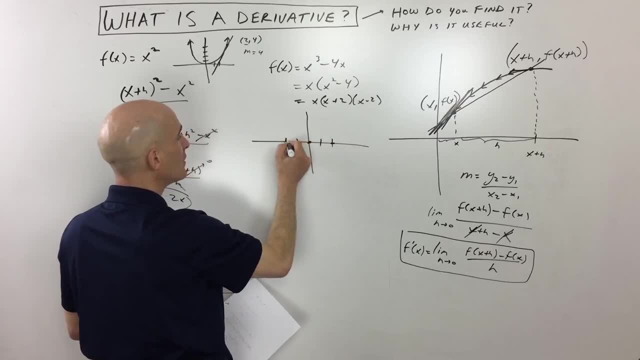 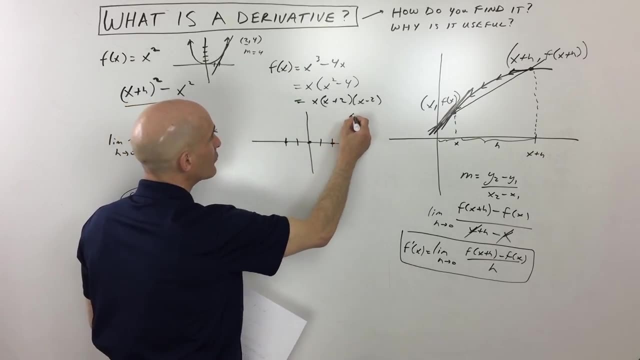 positive 2 if we set that one to zero and we're getting negative 2 if we set this group equal to zero And we know the leading coefficient's positive, okay, which tells us that the end behavior is going up to the right, and we know it's an odd degree, so that means it's going. 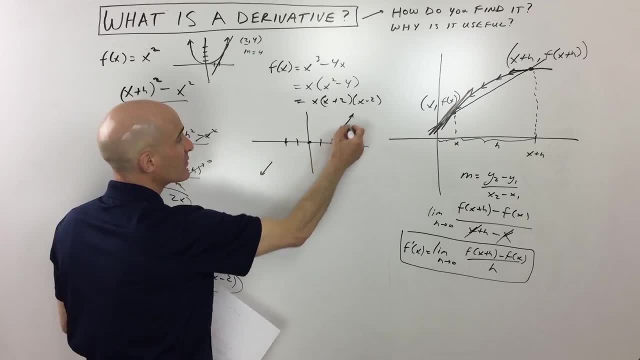 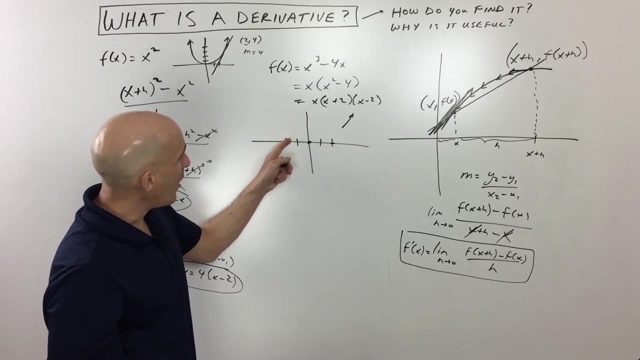 the opposite direction to the left, and we know the graph goes something like that through those points. But the question that students oftentimes have is, when you go through these points, like how high does that graph go before it turns around? Does it go way up here and then come back down? 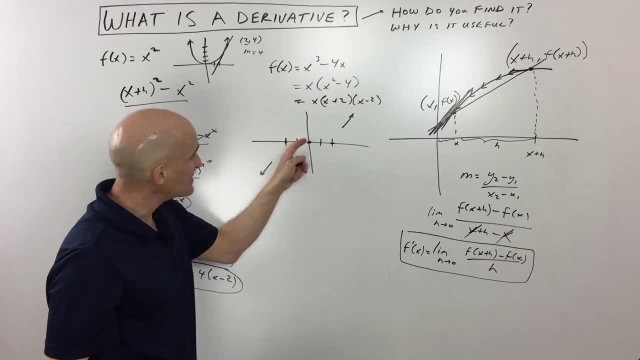 here and go. Does it go way back down here, or does it just go a little bit past the x-axis? You know how do we find that out, How do we find those turning points? Well, what's interesting is that when the graph 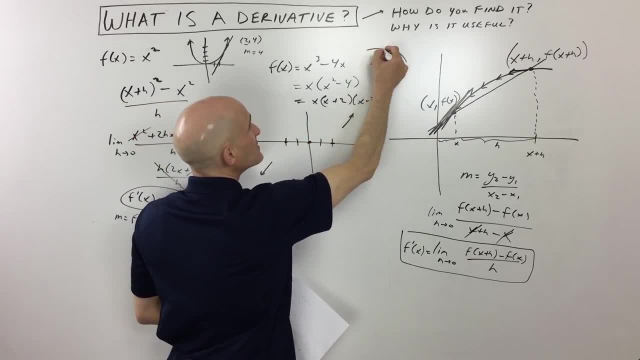 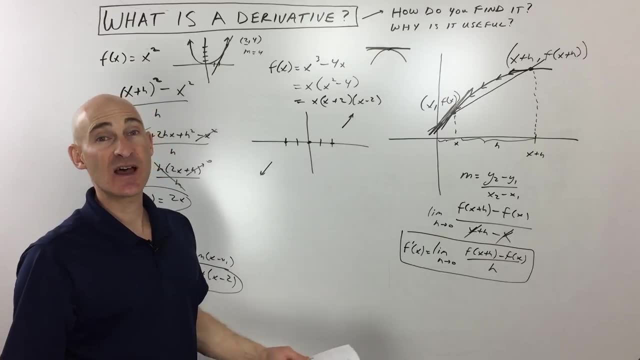 bends when it turns. okay, say, for example, like this: what's the slope of the tangent line at that point where it turns? Well, you can see, it's a horizontal line. so the slope of that tangent line is zero. So what we're going to do is we're going to find the derivative of our equation and we're 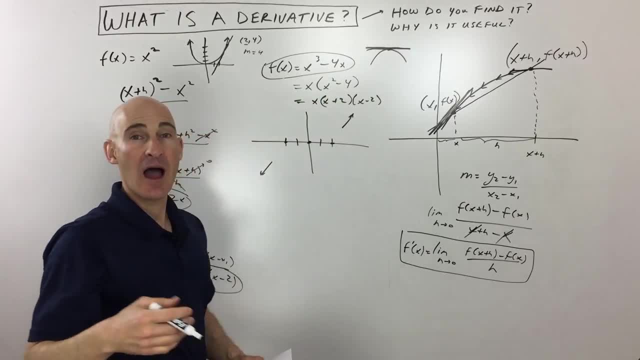 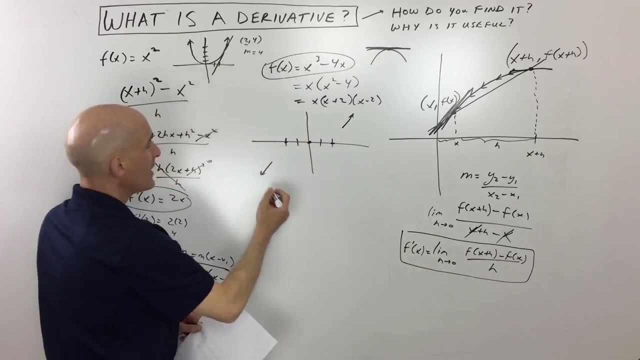 going to set that derivative equal to zero, so we can find the points on the graph where the slope of the tangent line is equal to zero. Okay, so we're going to use our difference quotient, again, our derivative formula, right here, and so let's do that. So we've got x plus h cubed minus 4 times x plus h minus f of x, which is this original. 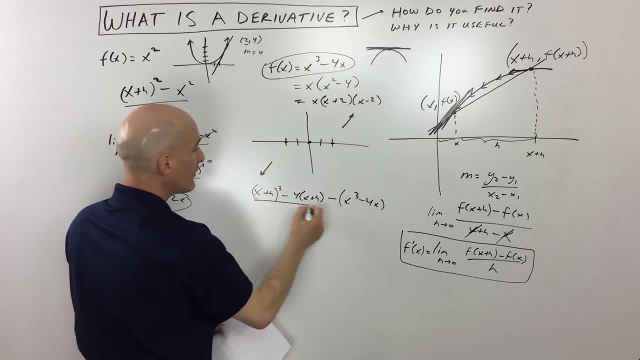 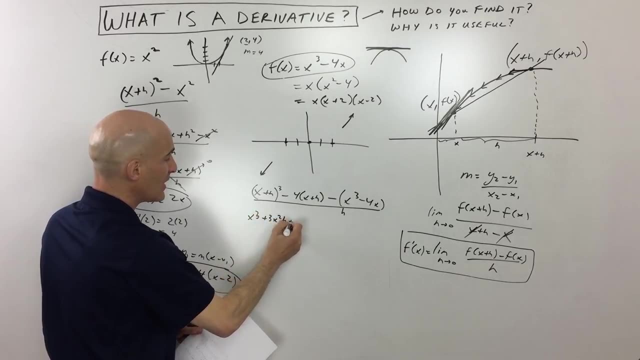 function. so that's going to be x cubed minus 4x, all divided by h. Okay now, if I simplify this, this comes out to x cubed plus 3x squared, h plus 3x h squared. I'm using the binomial expansion theorem. 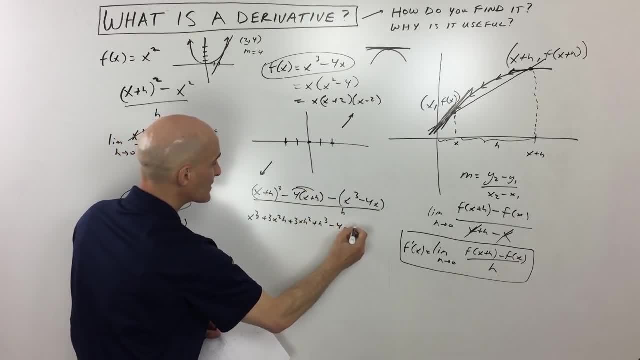 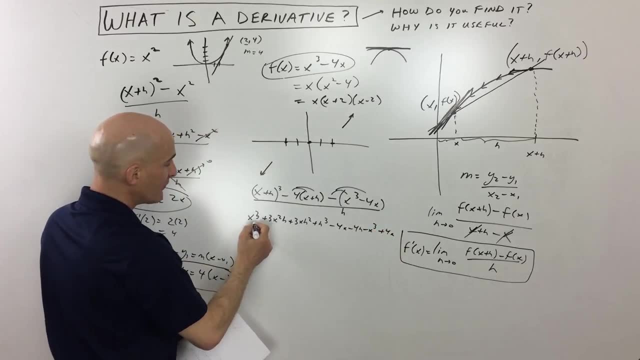 here. Distribute the negative 4, so that's negative 4x minus 4h. Distribute the negative here, that gives us negative x cubed plus 4x, and this is all divided by h. Okay, and you can see we get a lot. 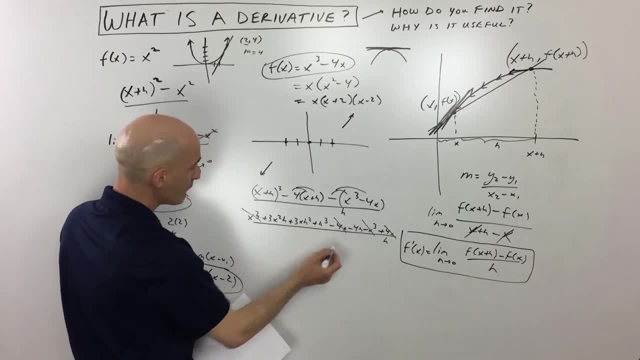 of cancellation: The x cubes are canceling, the 4x's are canceling, and then, if we factor out an h out of what remains here, we get 3x squared plus 3x, h plus h squared minus 4, all divided by h. 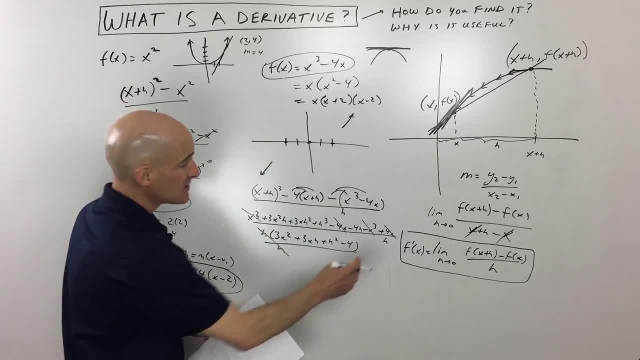 You can see those h's are canceling, But remember it's the limit as h approaches 0, right, So if we put 0 in now for h, this whole term is going to go to 0,. this whole term is going to go to. 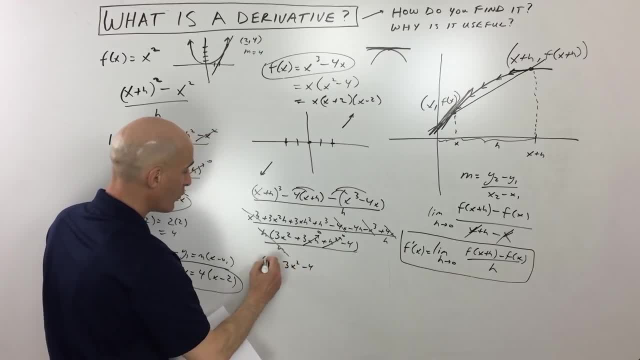 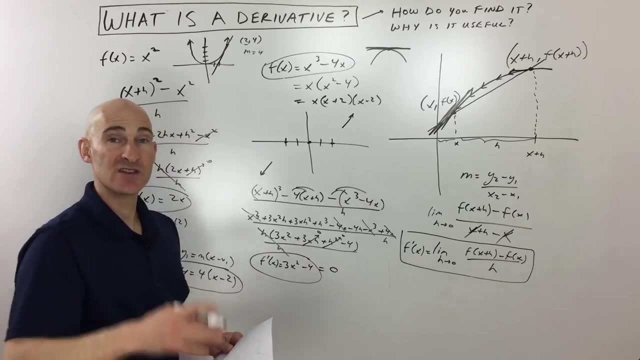 0, and we're left with 3x squared minus 4 is our derivative. Okay, that's a formula for our slope, but what we want to do is we want to find out where that slope is 0.. Okay, that's where the graph is. you know turning around or bending, and so what we're going. 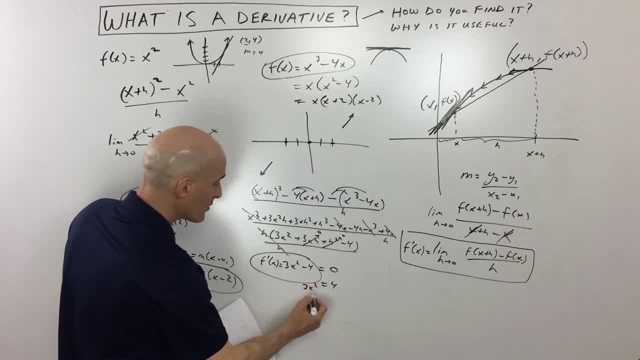 to do is we're going to add 4 to both sides. Okay, so that's 3x squared. We're going to divide both sides by 3, so that's 4 thirds. We're going to take the square root of both sides. 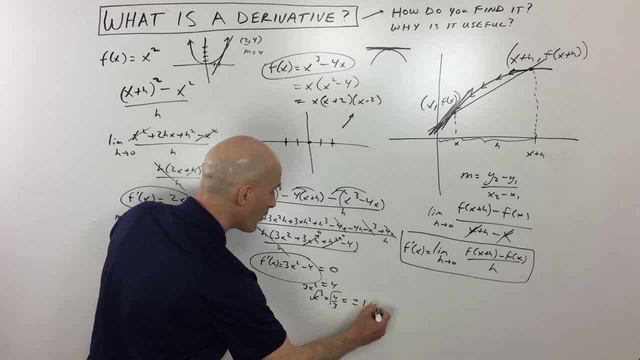 That gives us plus or minus, and I did this on the calculator. for us it's 1.15,. okay, Now if we put 1.15 back into our original equation, what we get is 1.15 comma negative 3.08, and if we put in negative 1.15, we get positive 3.08.. 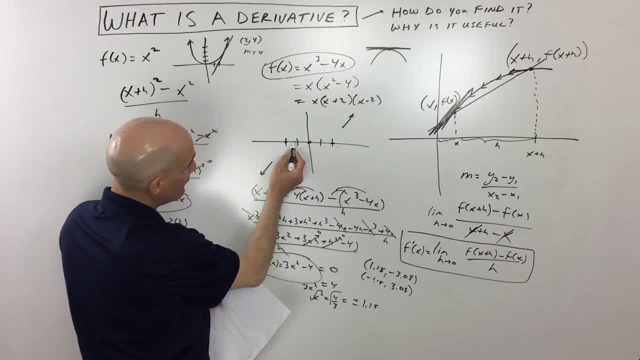 So those are our turning points. So if we graph this, you can see at negative, 1.15, we're going to be up here at, let's see, we're going to be at 3.08, so it's going to be right about there. and if we're at positive, 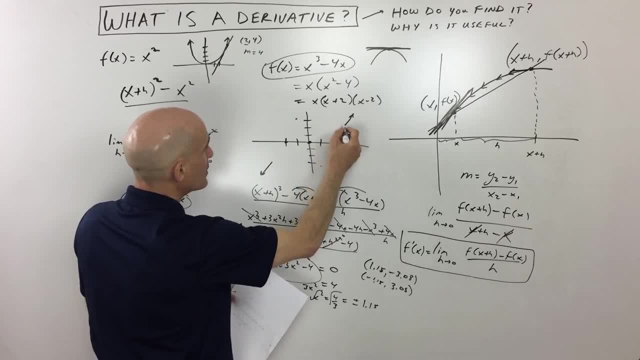 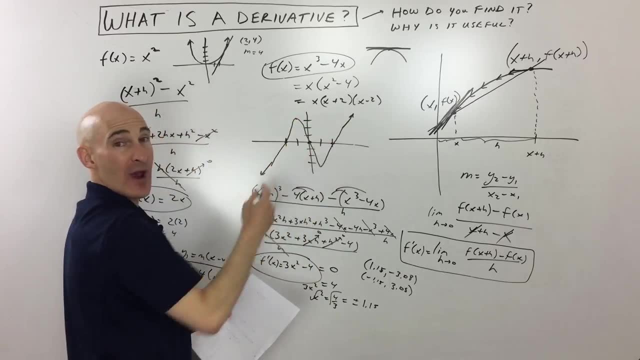 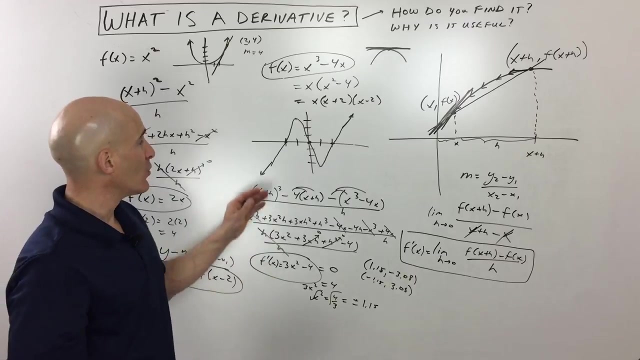 1.5, we're going to be right about there. So that gives us a better idea, okay, of how high the graph is going and how low the graph is going. Otherwise we're just kind of guessing. We don't really know where those extram are, those maximums and those minimums, right? 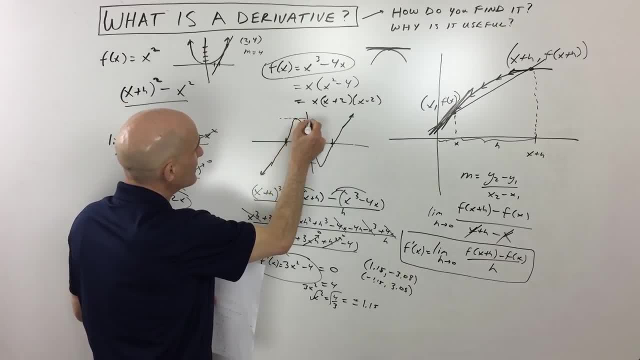 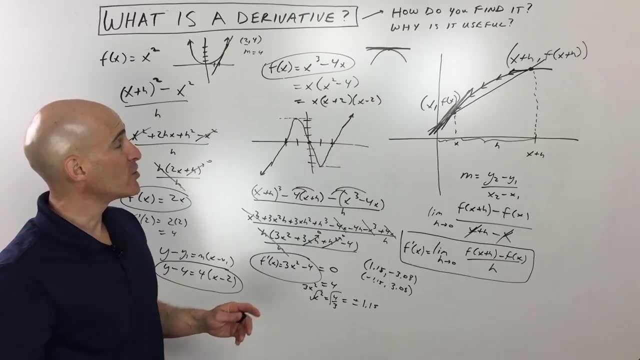 So that's a key point. And again, you can see that. You can see where that graph is bending or turning or changing direction. That's where the slope of the tangent line is equal to zero. So key points to remember when you're learning about derivatives is: you know what is a? 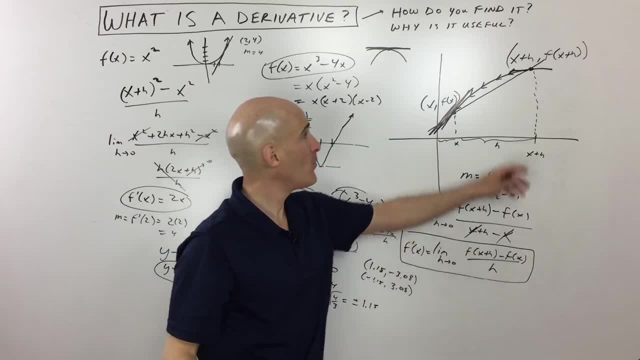 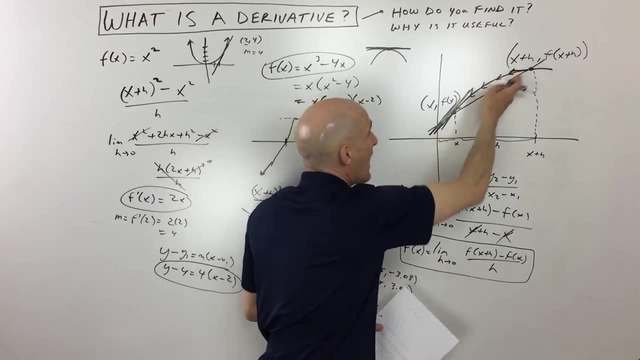 derivative. It's really a formula for the slope. How do we find the slope? We take these two points, okay, and we use our slope formula. but we take it a step further to go from the average rate of change to the instantaneous rate of change by using limits. 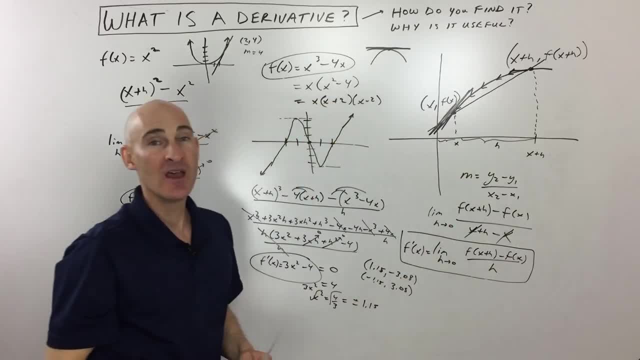 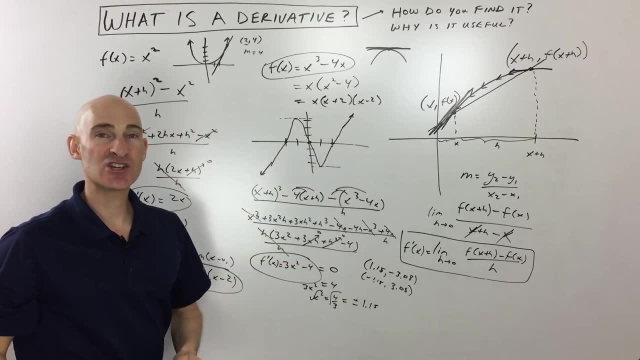 and the limit as h gets smaller and smaller, It approaches zero And then from there, once you have the derivative, you have a formula for the slope of the tangent line and you can- you know- use it in some of these applications like we talked about.